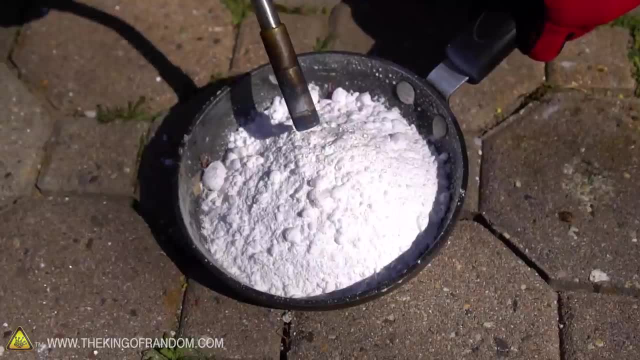 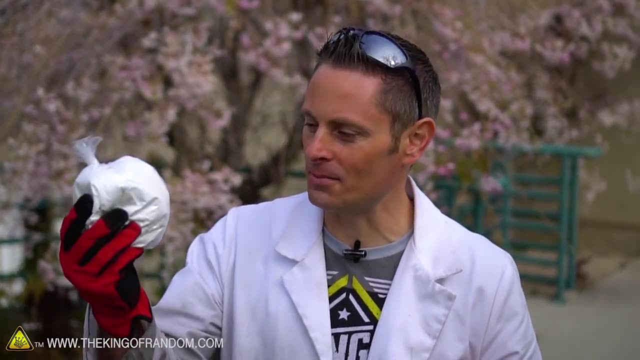 Instead, if we can throw enough heat at it, we can actually get it to melt down, because it's actually got a melting point around 672 degrees Fahrenheit. So this is the purpose of our experiment today: Let's melt down our potassium chlorate into a hot molten bath. 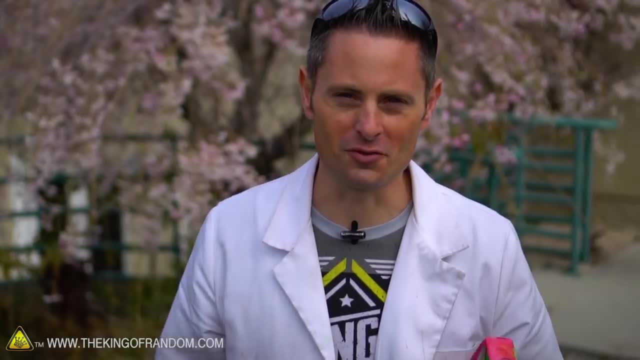 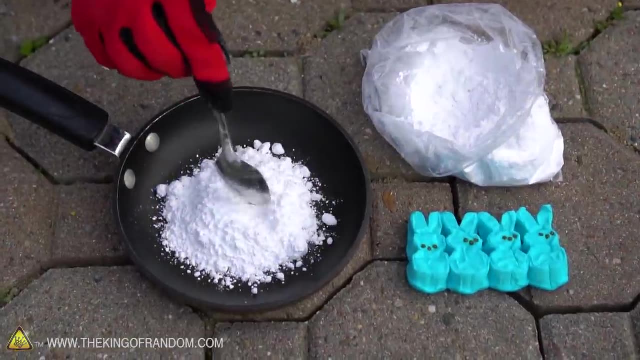 then take one of our little marshmallow peeps and let them go for a swim and observe what happens. It really looks and feels a lot like powdered sugar. That should be more than enough. So quick update on what I'm thinking here, guys. 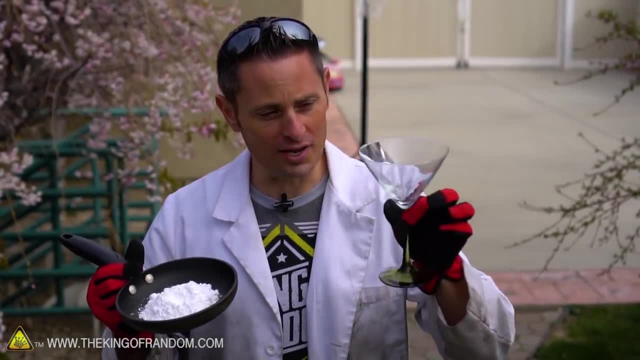 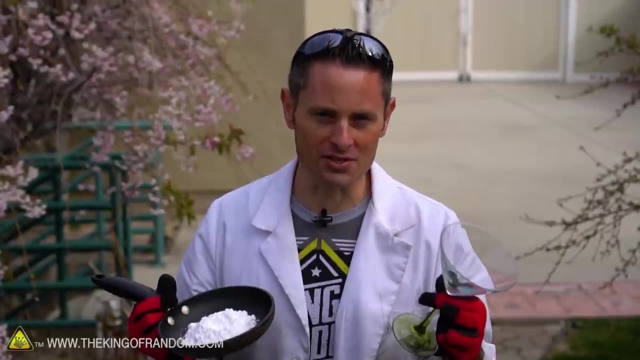 We're going to get this stuff up to about 700 degrees Fahrenheit, and I'd really like the reaction to take place inside of a glass. Now the problem is glass is sensitive to thermal shock, and if we take a blowtorch to it it'll probably shatter into a million pieces. 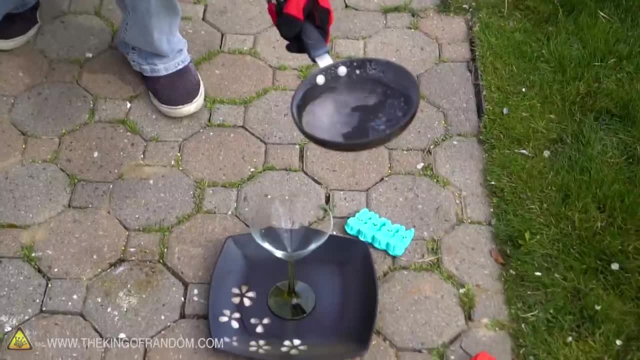 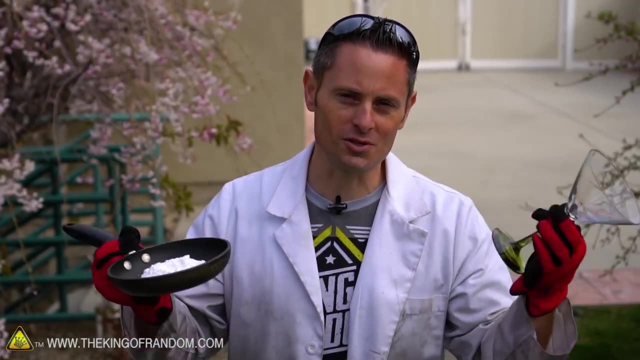 So what I'm hoping we can do is liquefy the potassium chlorate in the pan first and transfer it slowly into the glass, where it may have a little bit better chance of staying intact. If it does, we should be good to go, and if it doesn't, we'll just find another way. 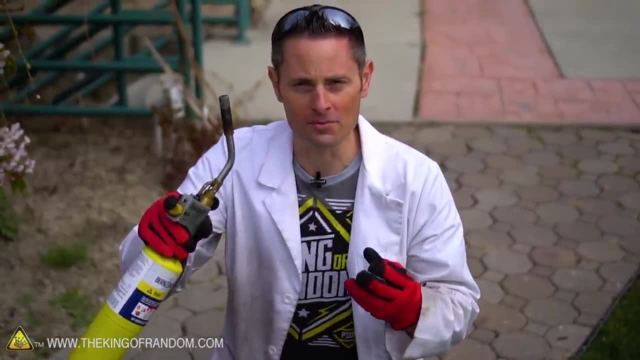 I'm using a map gas torch which produces a very, very hot flame, so I'm just going to sweep that back and forth over the white powder until it liquefies- And I've never actually liquefied potassium chlorate before. 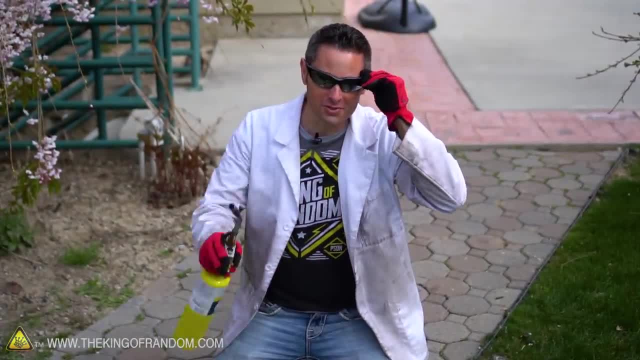 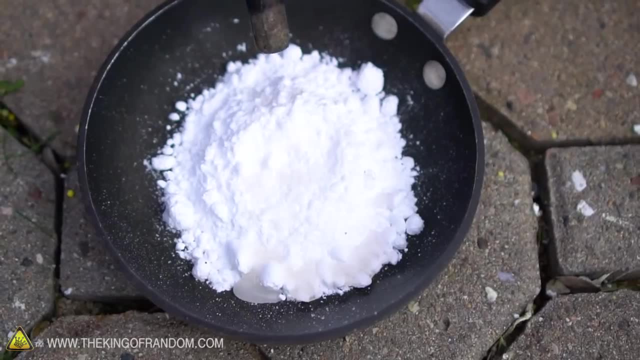 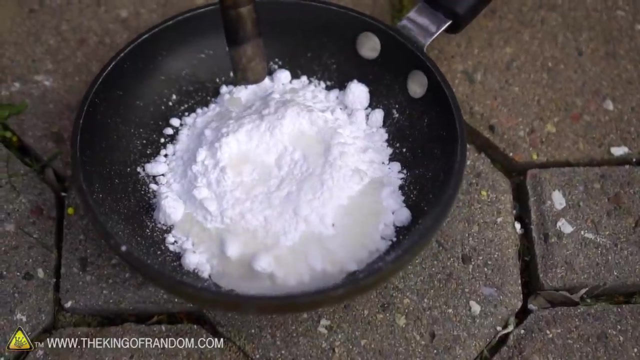 so I'm very interested to see how this looks. Glass is on for safety. Let's rock. There we go. You can actually already see at the top there parts of it are liquefying and melting down and the edges here are spewing. 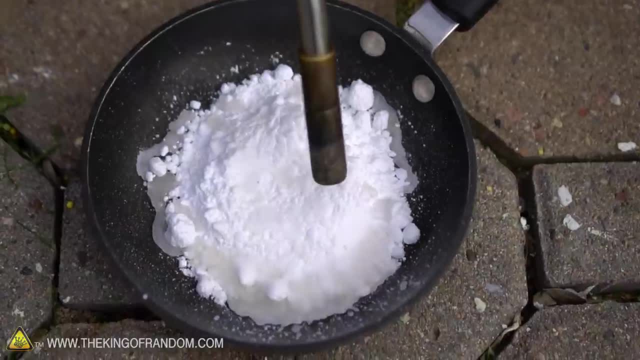 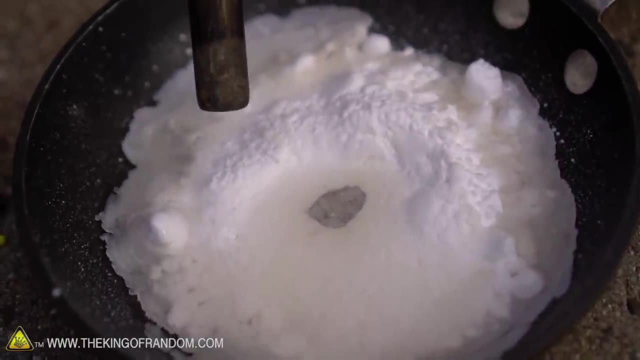 It looks like they're reacting with something. Maybe that's the nonstick surface of the pan itself- Not exactly sure, But it doesn't look like it's taking too much to melt this down. It's definitely a different reaction than if you were to try this with sugar. 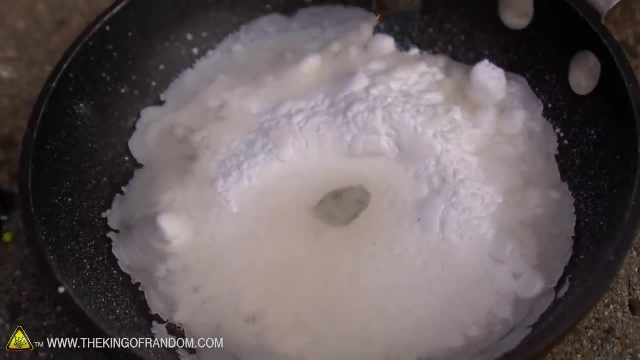 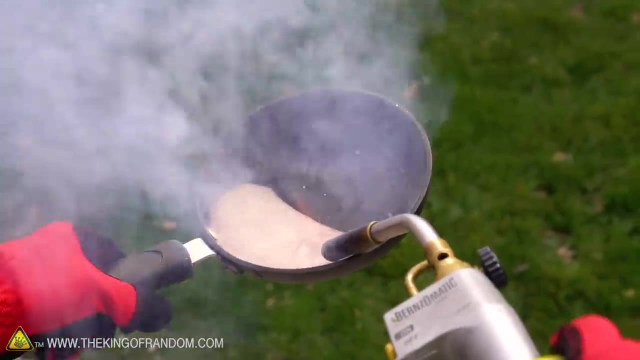 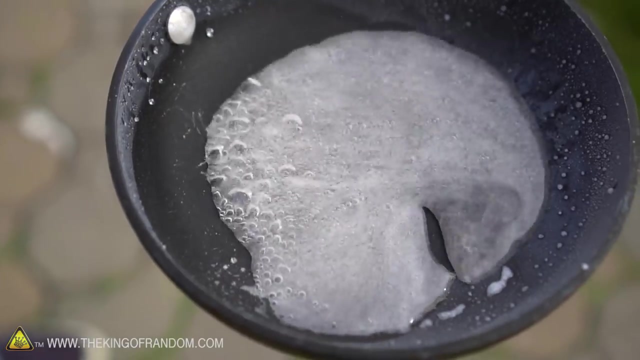 The sugar would just burn and turn black. But you can see this is turning into a very translucent liquid syrup. It's not sticking anymore. That's a good sign. Our potassium chlorate is completely molten now. It's not even sticking to the pot anymore, so let's go ahead and transfer it to glass. 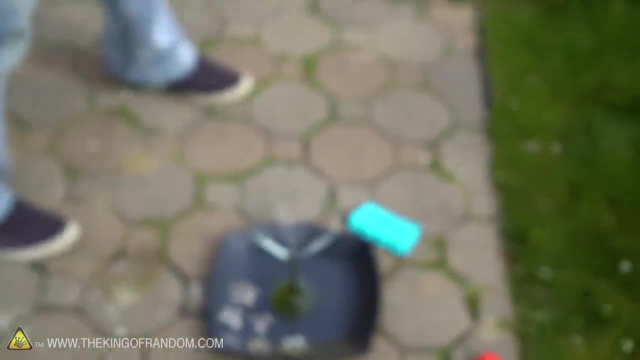 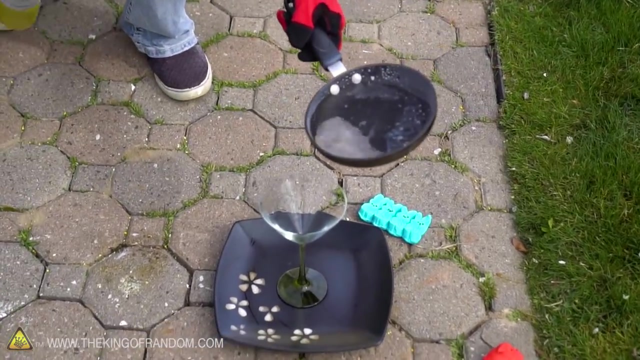 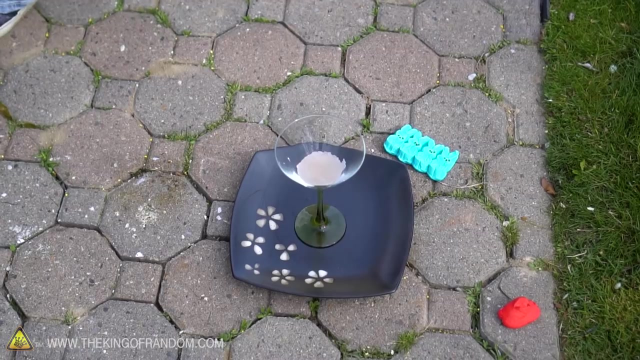 My only concern is whether or not the glass will hold up. There's a possibility it'll just crack and splatter this stuff everywhere. Get that glass warmed up a little bit Very carefully. make the transfer Cool. Holding up so far. 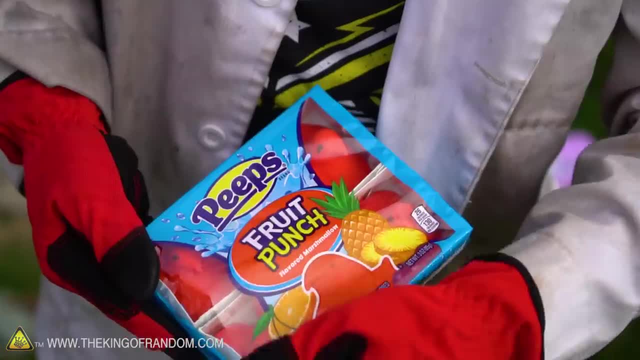 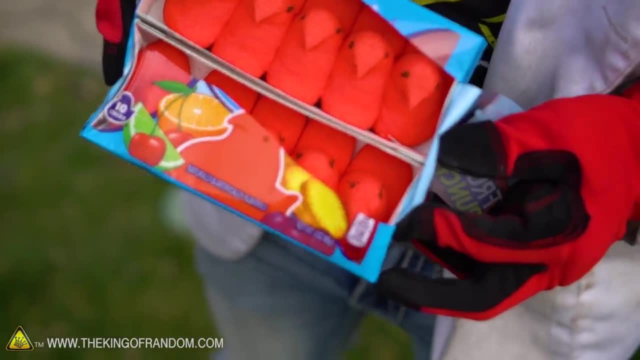 Now that we've got our potassium chlorate completely liquefied, let's take one of our fruit punch flavored peeps and let them go for a swim. Ooh pretty, Oh, this one looks like he's crying. Oh, don't worry, little buddy, It'll be over soon. 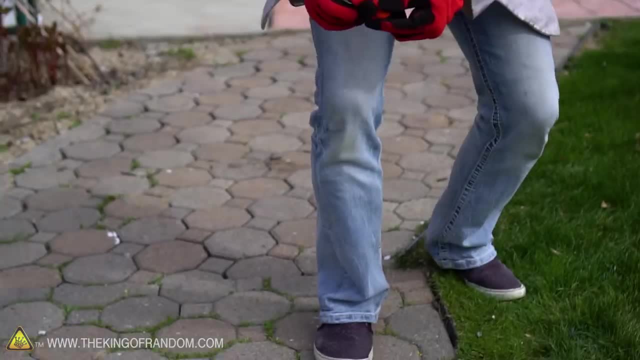 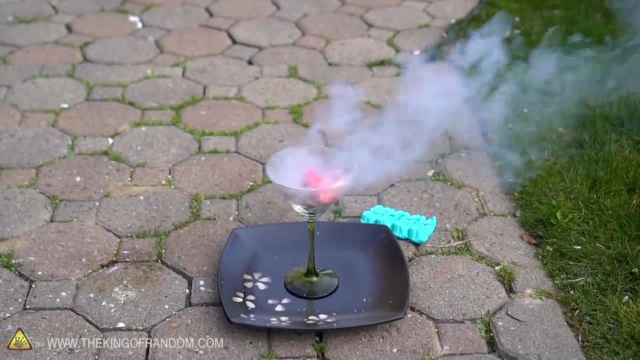 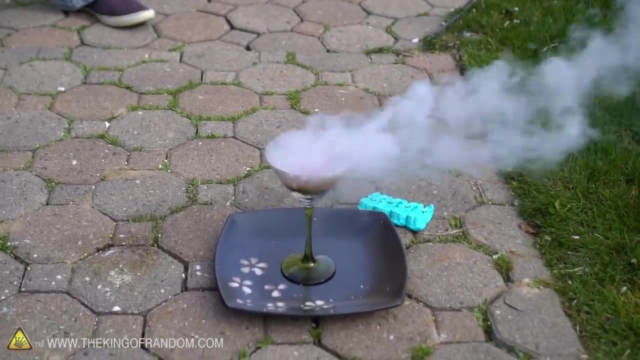 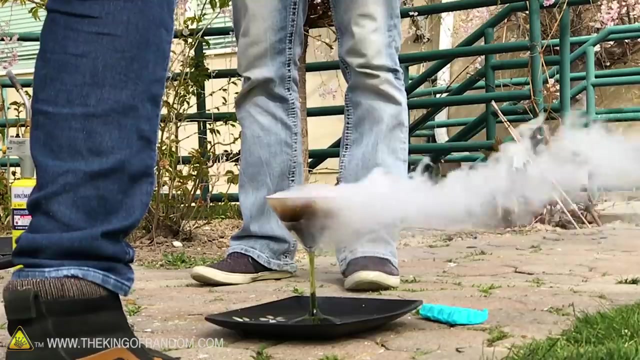 That's so wrong, isn't it? What's gonna happen? What's gonna happen? Three, two, one. Oh my goodness, Oh my goodness. Oh, there goes the glass. That is crazy. I can't believe how quickly that took off. 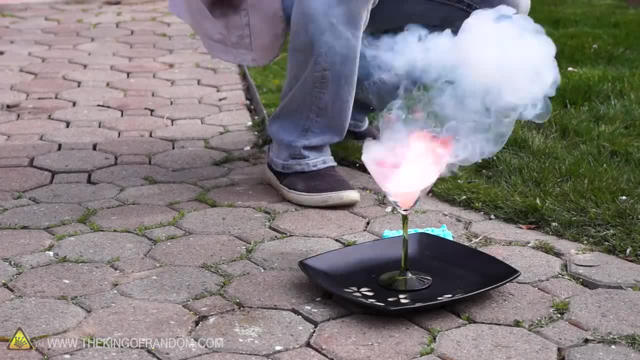 It was like instant reaction: Just burst right into flames like the second it made contact. Just burst right into flames like the second it made contact. I don't have enough time to get my hands away, Guys. you gotta come check this out. 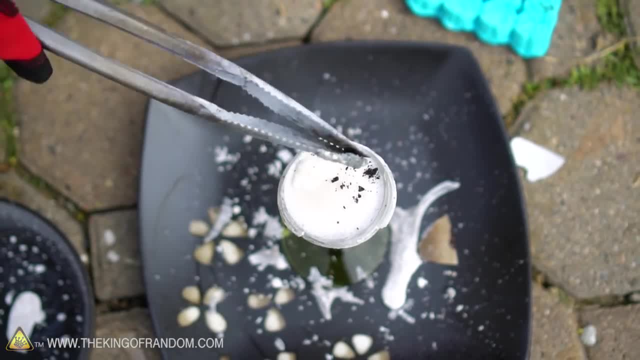 There is nothing left of that red peep. Look, It is completely disintegrated. All that's left is a little tiny bit of black ash residue. All that's left is a little tiny bit of black ash residue, But other than that it is gone. 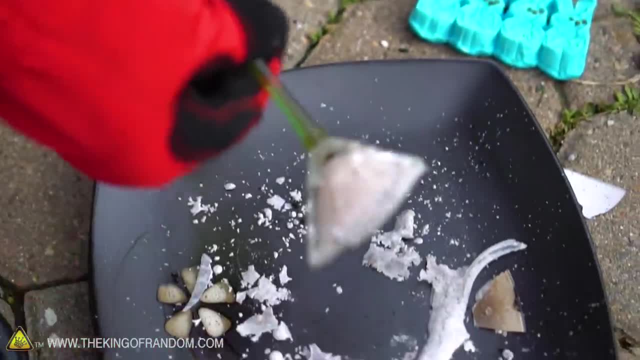 And you can see our potassium chlorate has actually solidified again back into this big white blob. And you can see our potassium chlorate has actually solidified again back into this big white blob. Whoop, there it goes, Oh sweet. 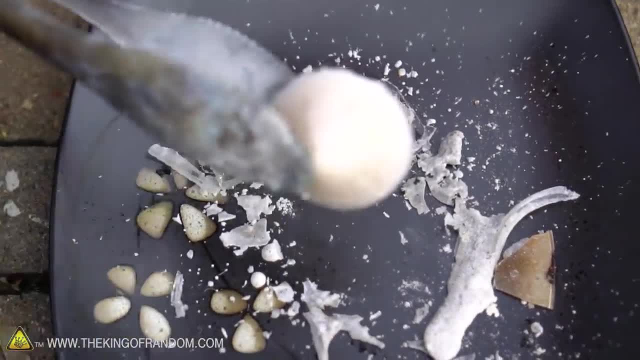 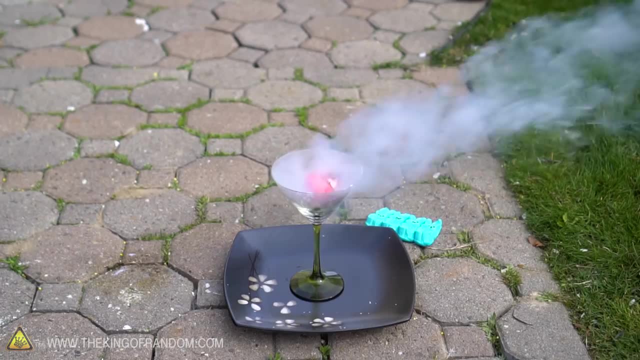 So it looks like this stuff is castable. Look at that. I just cast it into a cone shape. That's kind of fun. That reaction took off immediately. It went into these bright magenta, pink flames, Very, very vigorous, and produced a lot of smoke. 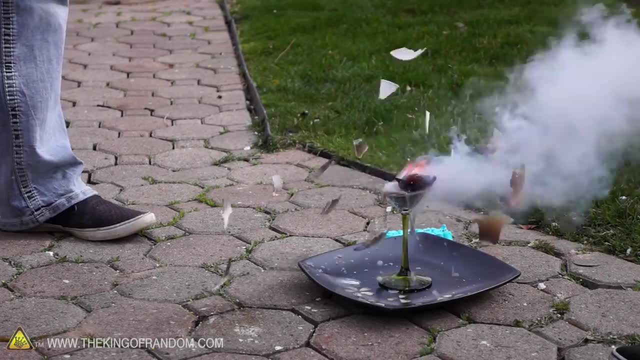 That was pretty cool. And you can see from the heat of the reaction the glass actually did end up exploding everywhere. And you can see from the heat of the reaction the glass actually did end up exploding everywhere, Which is why I put this plate underneath it, so we can recapture some of the potassium chlorate and use it again. 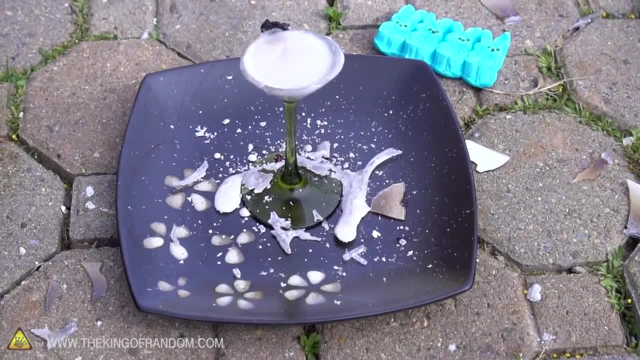 Which is why I put this plate underneath it, so we can recapture some of the potassium chlorate and use it again. It's expensive stuff, you know. For our next experiment, I thought it would be fun to try one of these decorated marshmallow Easter eggs. 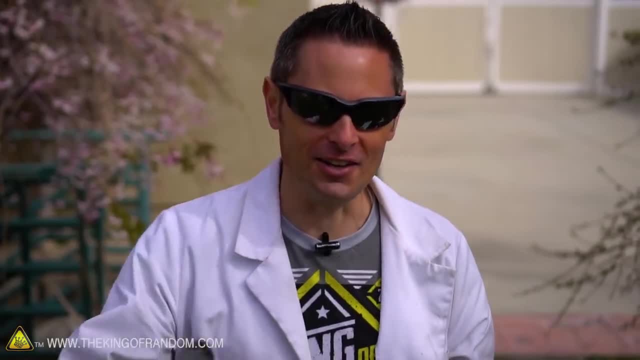 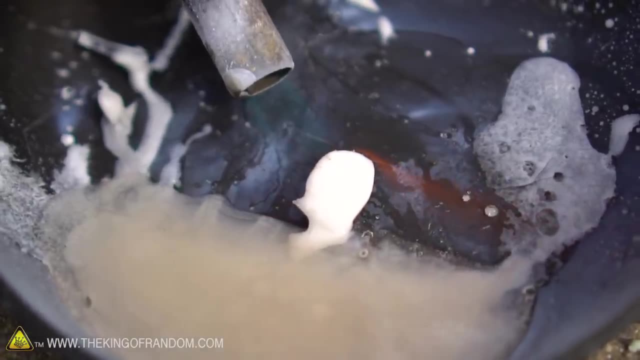 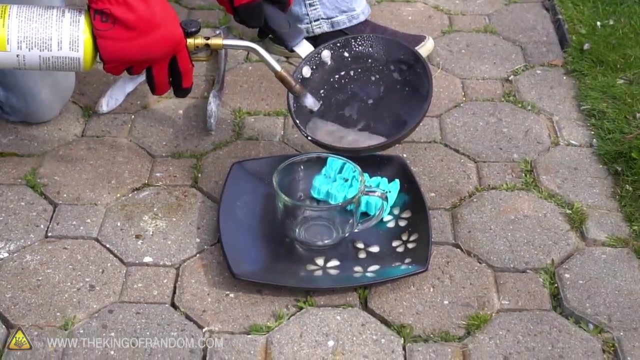 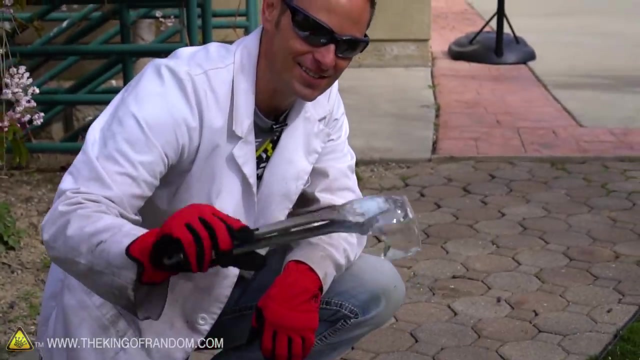 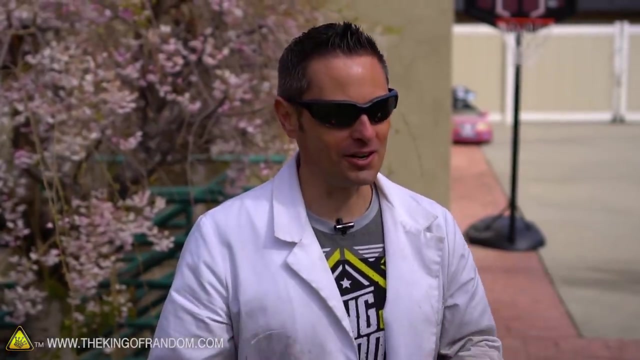 So let's recapture some of our potassium chlorate, melt it down and light it up. oh, there goes the glass. look at that. that glass is done. so you get for getting your glass at the dollar store, okay, so that was kind of expected when i poured the potassium chloride into the. 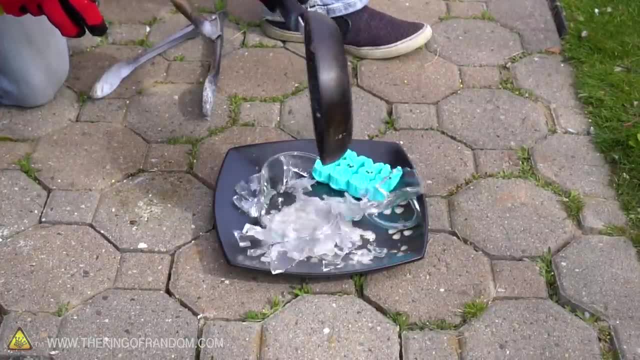 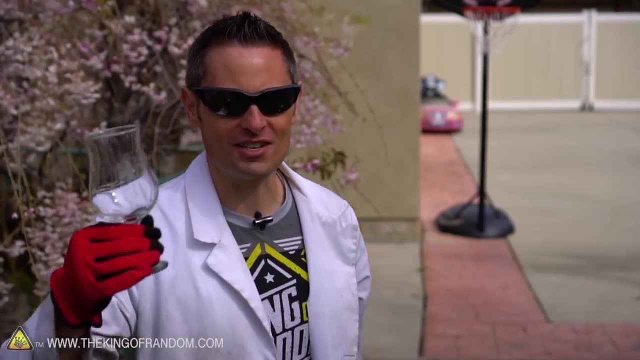 glass. it sat there for like just a couple of seconds and then completely shattered. it's because it wasn't able to withstand the thermal shock. we're down to our last glass here. i'm not very confident it's going to hold up either. let's go ahead and put it to the test. 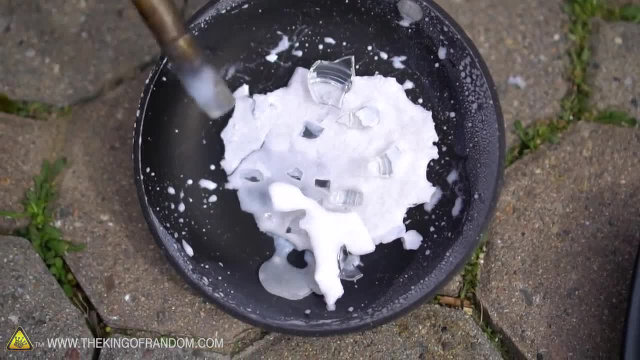 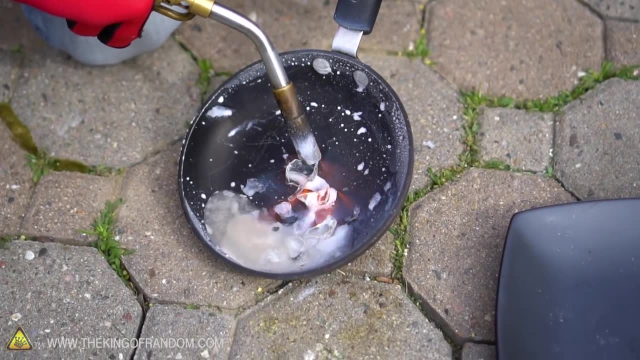 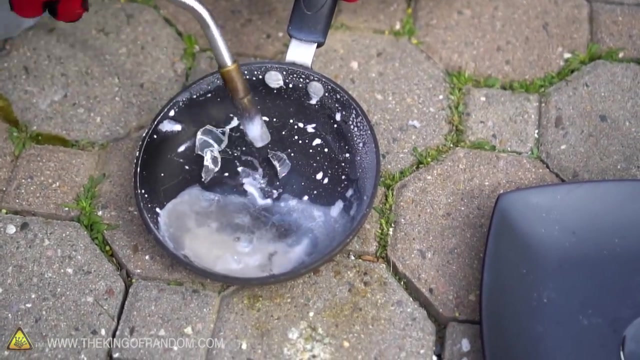 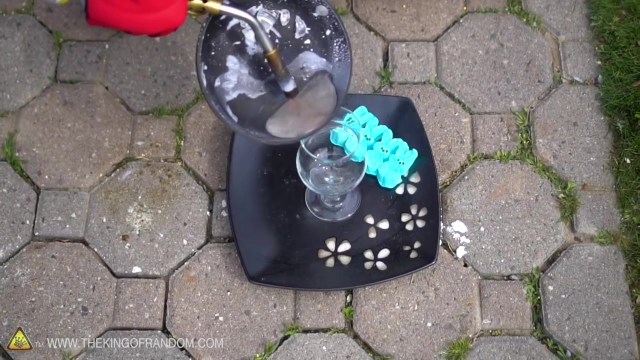 anyway. you can see there are chunks of glass still stuck in there, but those are going to come right out in the solution. you can see how those glass pieces are free- now freedom- and you separate them right out. will the glass survive? here we go all right. so far, so good. let's go ahead and throw in our egg. 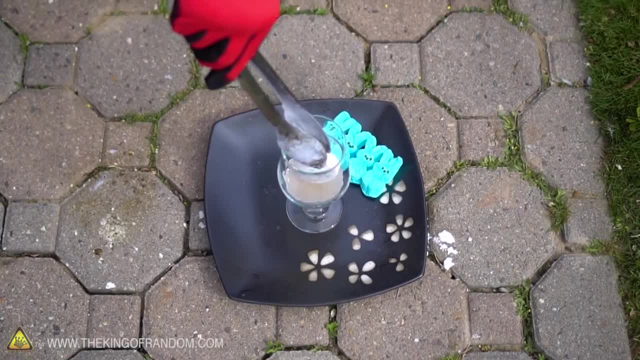 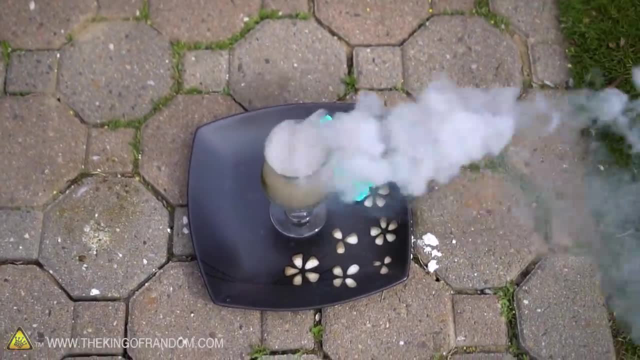 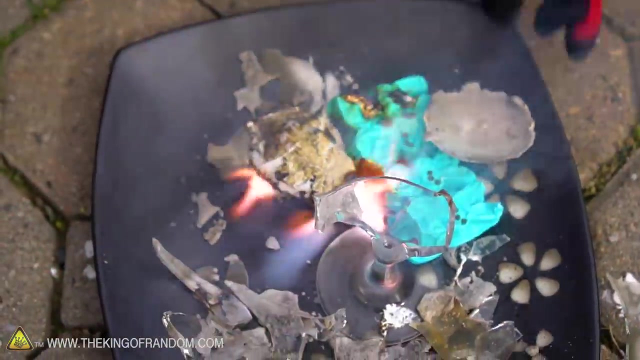 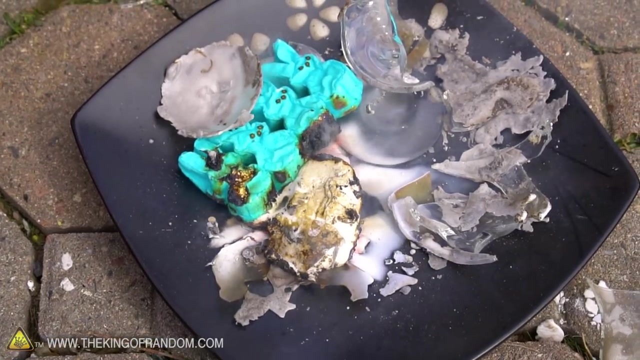 i'm gonna be a little bit gutsier now that i've got the tongs here, here we go and contact whoa. look at, i was gonna say look underneath there, look at the color of those flames. see how you got like beautiful magenta, pink, some orange in there. so as much as i wanted to do these- 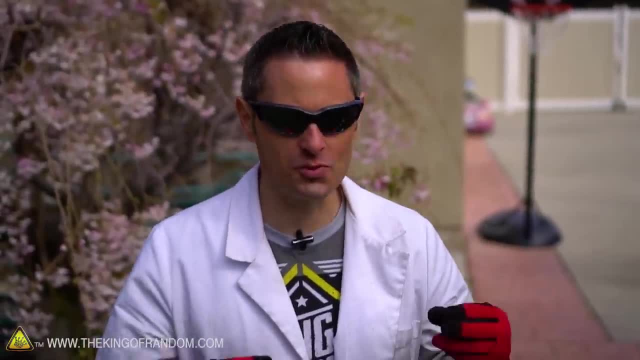 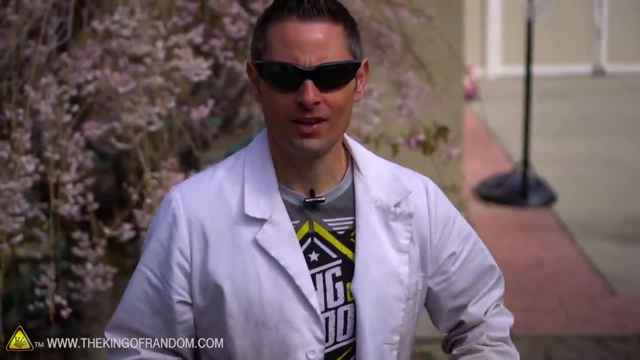 experiments in glasses. they're not holding up very well to the heat. you can see that just within a few seconds of pouring the molten potassium chloride, oh there goes, the plate plate just cracked. so as much as i want to do this reaction inside of glass containers, they don't hold up very. 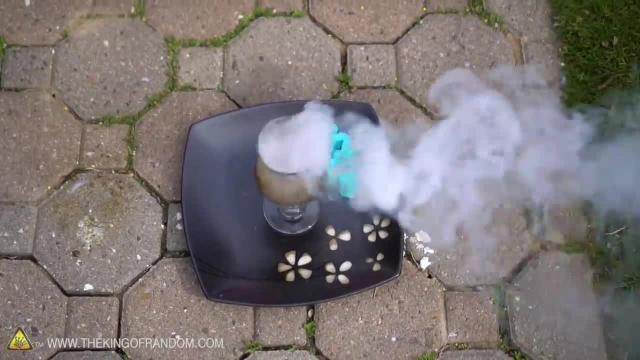 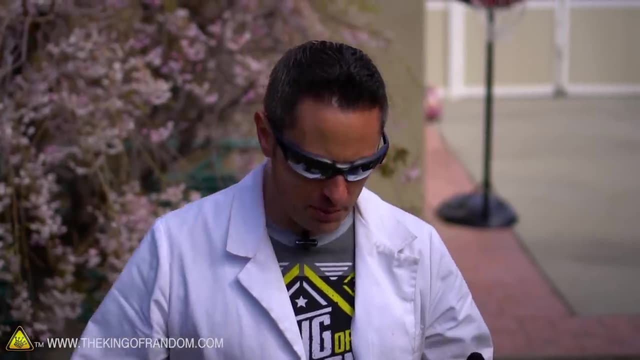 well to the heat at all. you can see that within a few seconds of the liquid making contact with the glass, it shatters and spills out the molten material, and then it very quickly solidifies and the reaction stops. so for our next experiment, let's try placing our peeps down below and 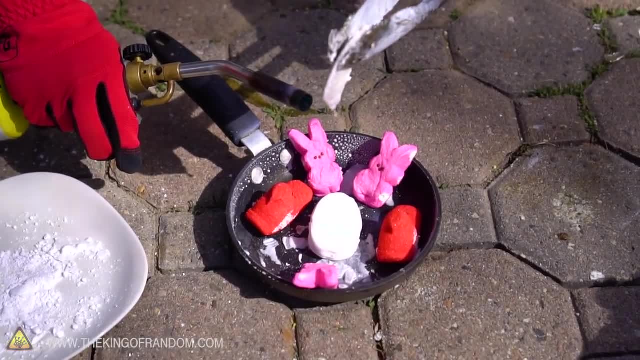 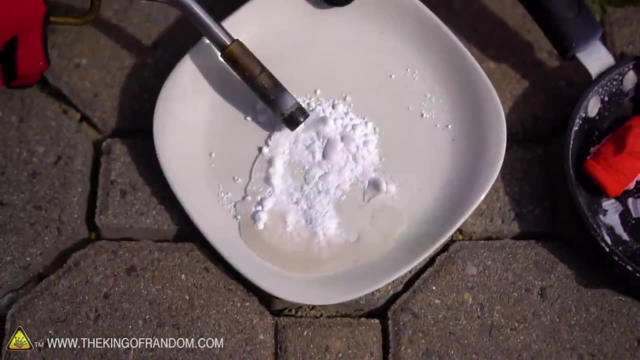 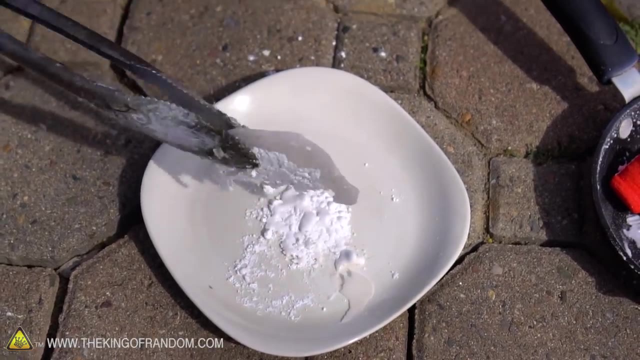 melting the potassium chlorate from above, so it drips down out of the marshmallow- and watch what happens in that scenario there and i'm just going to let that cool down and solidify should give us a nice little chunk that we can go down to. so here we are. i've got a nice chunk of our chlorate melted down. 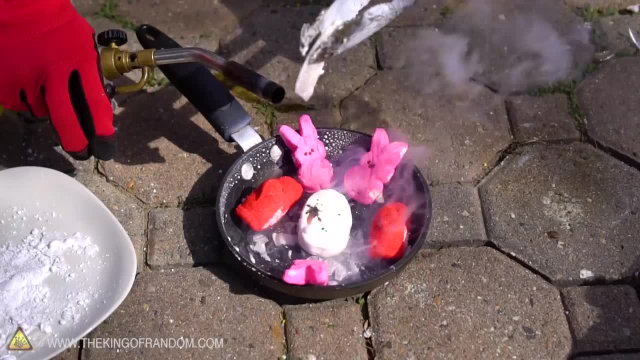 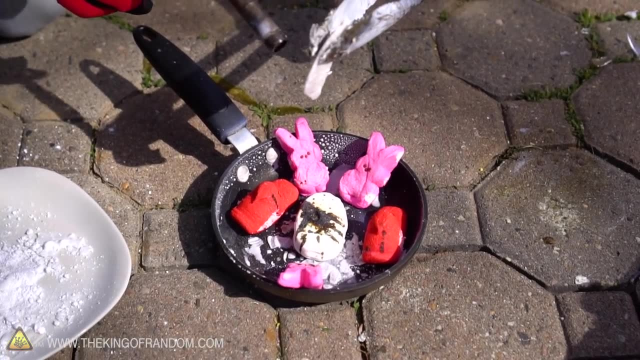 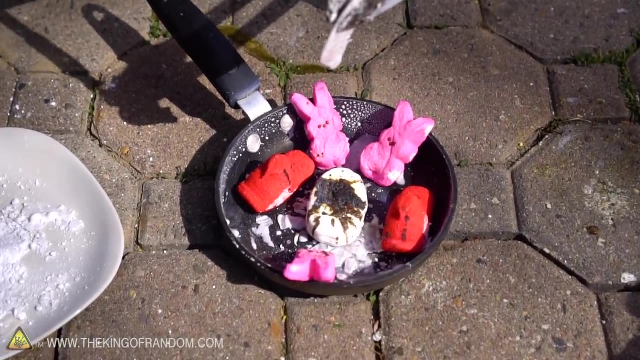 and re-solidified. now we're just going to hold the flame to it and drip it down onto our peeps. oh, that's so cool. you can see how it balls up on the top and then just explodes- boom. this stuff drips off, and when it hits the marshmallow it has such a vigorous. 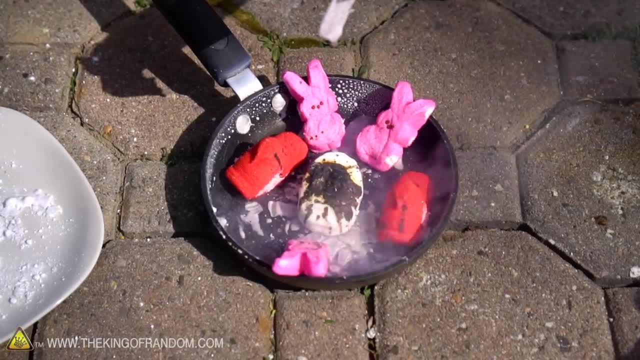 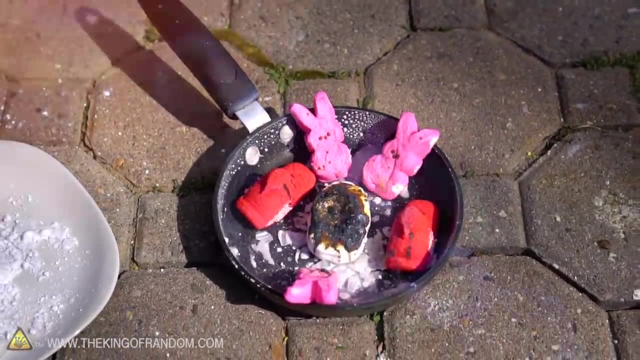 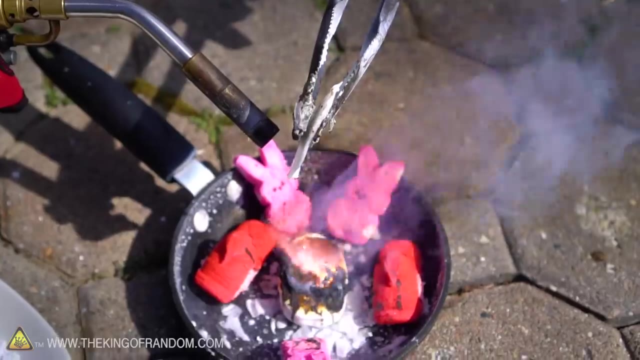 reaction: it just explodes. sweet, let's do that again, but a little bit longer. what we saw in that last experiment was a lot more stability and control, because we were able to regulate the flow of potassium chlorate down onto the peeps themselves. when the stuff actually hit the peeps, it seemed to ball up into a very vigorous reaction and then explode. 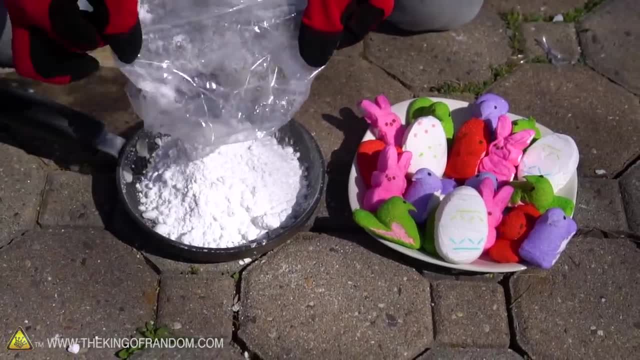 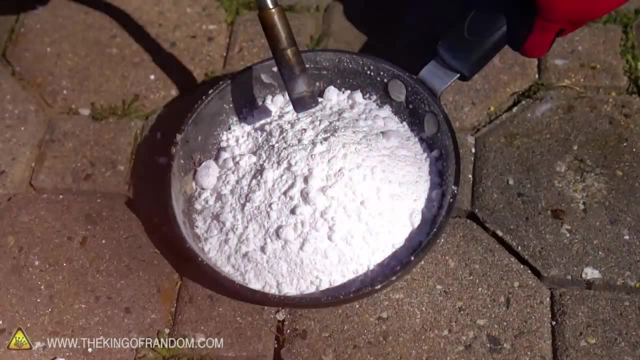 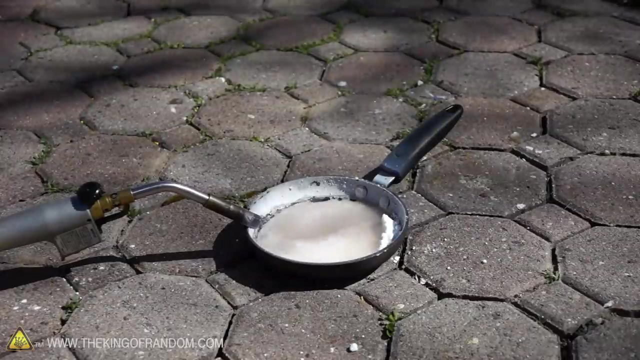 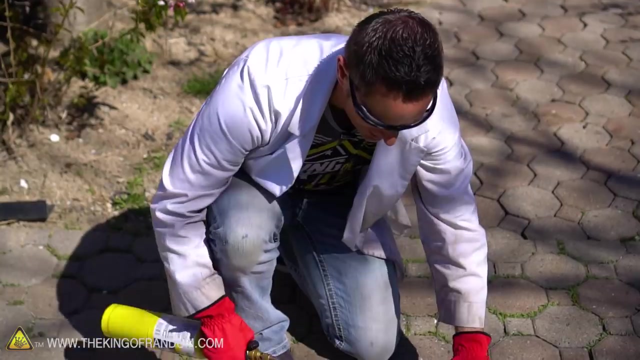 for one final experiment, let's mix up one large batch of molten potassium chlorate in the pan itself and take a whole peep party and throw the whole lot in at once. that's so cool, huh? look at that, guys. we have a huge pot full of molten potassium chlorate. let's get ready for the big. 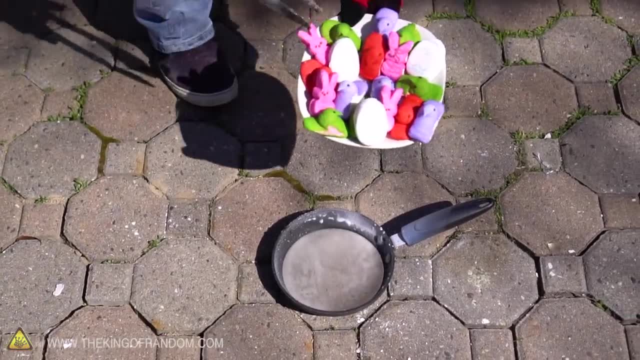 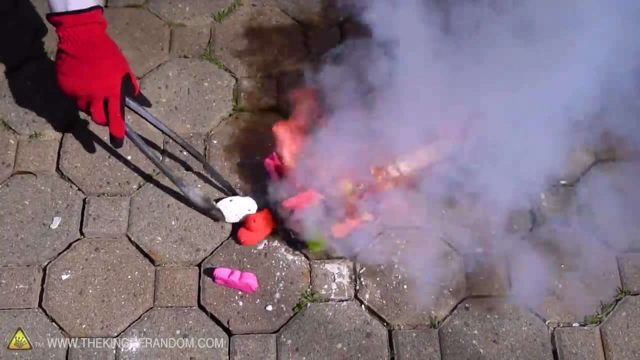 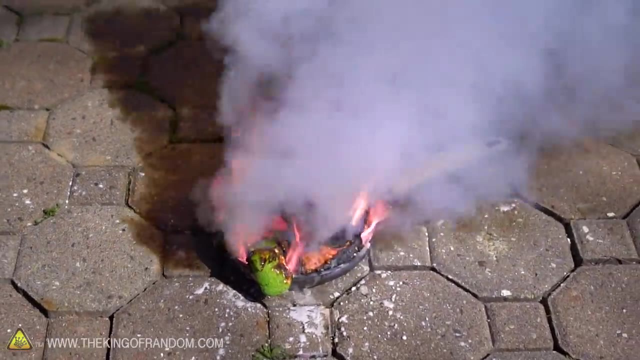 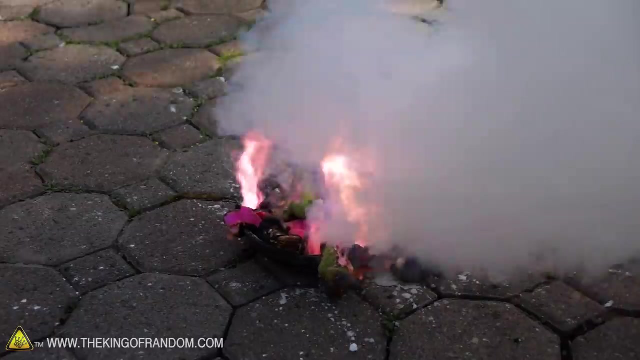 finish, let's do it. peep, peep, peep. we don't want these guys to be left out of the party. the smoke coming off, that's incredible. and look at those flames. we've got magenta, we've got pink, we got kinda like purplish whitish flames going on in there as well. 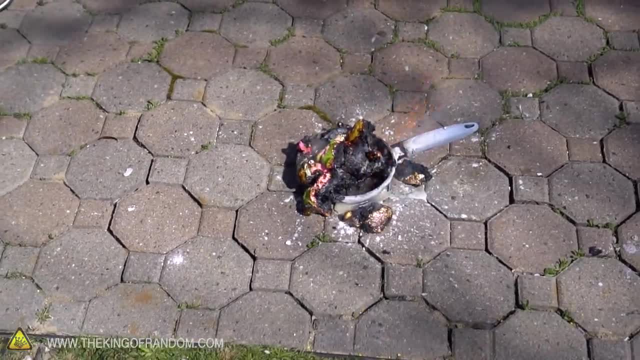 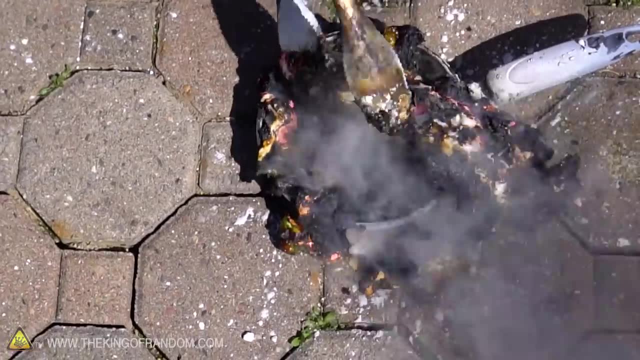 and the reaction just died out. Does that mean we used up all the of the heat in the first second? I hear it such aíe lies down up all of our potassium chlorate that quickly, What? Or did it just solidify And look yeah? 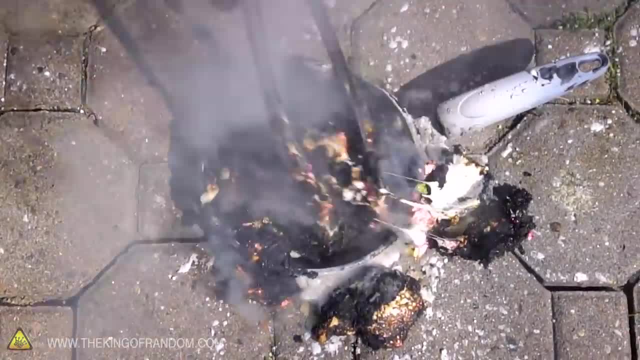 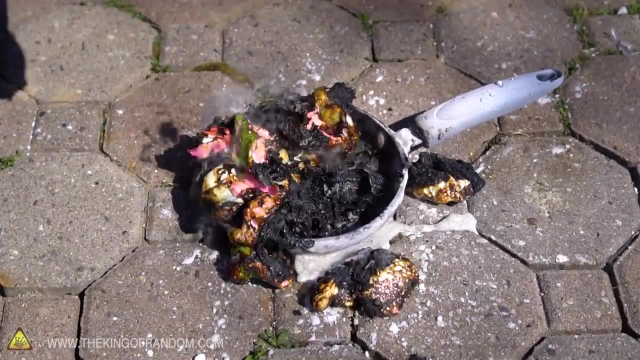 All the potassium chlorate is gone. That's amazing That burned up so fast. Look at that goopy gluey mess of molten peepee marshmallows. This one's still growing. Look at that. That looks pretty trippy. Check that out. These marshmallows are still on fire, though from. 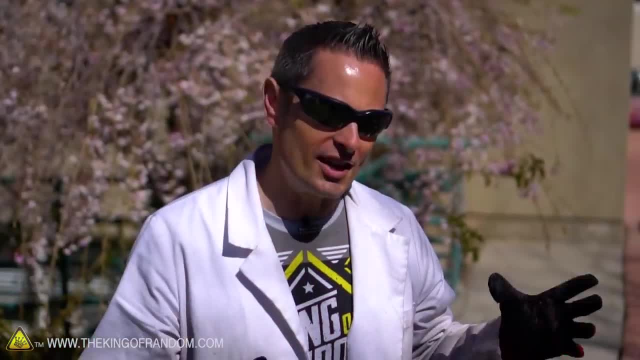 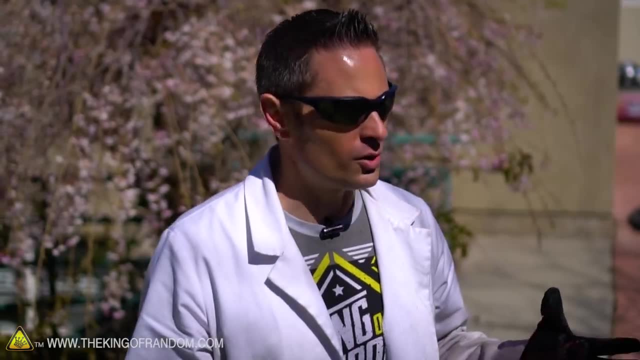 the heat of the reaction. Let's stop and take just a second to recap what we did here today. We learned about a chemical called potassium chlorate that's used as an oxidizer in building fireworks. It's normally a crystal or a fine white powder, but if we get it hot. 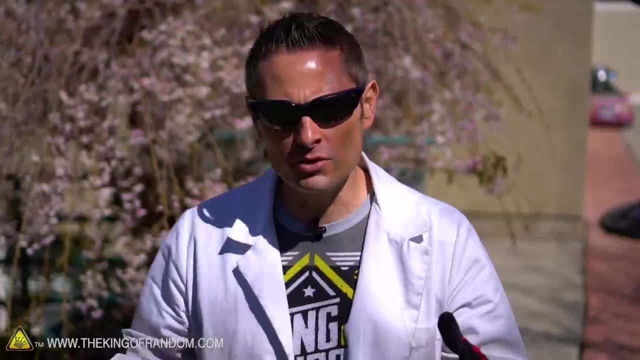 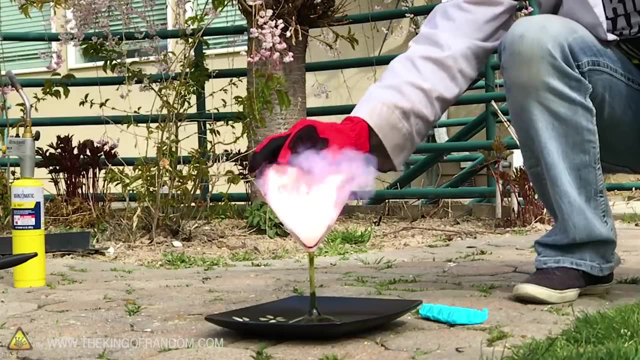 enough, it'll completely liquefy. We found that if we mix this molten potassium chlorate with peeps, it bursts into a very vigorous reaction of pink, purple and magenta flames- Very appropriate for Easter. We also found that the liquid is so hot that if we pour